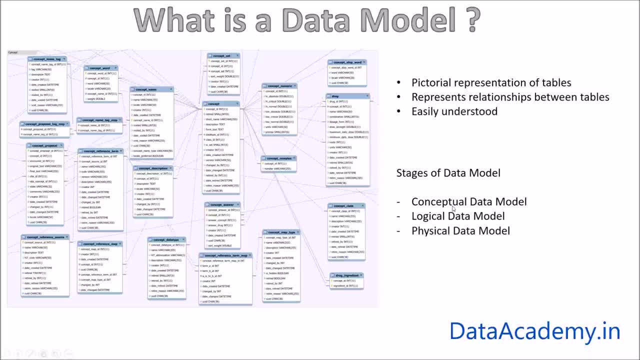 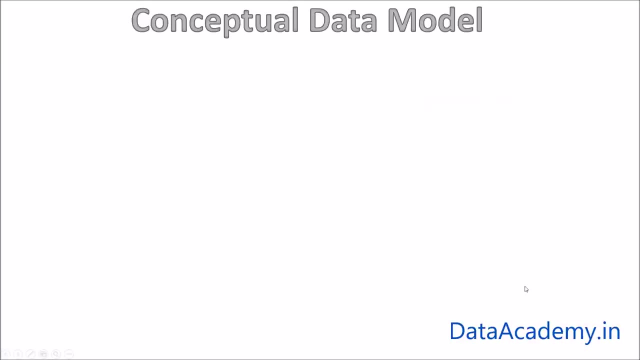 we progress through three main stages. They are conceptual data model, logical and physical data model, in this order. First, let's look at the conceptual data model. A conceptual data model is just a set of square shapes connected by a line. The square shape represents an entity and the 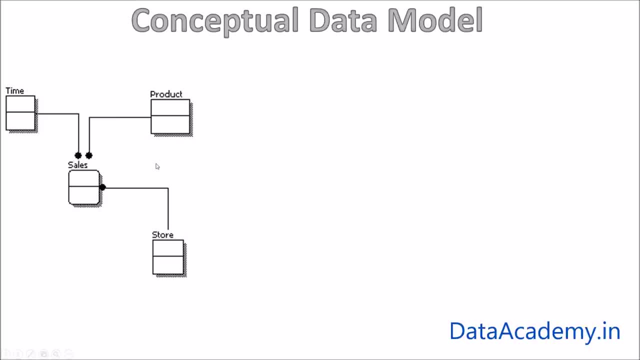 line represents a relationship between entities. A conceptual data model can be easily drawn, whiteboard or a piece of paper. it need not be a digital document. this makes it easy and quick to change and can be rapidly updated. so what are some of the attributes of a conceptual data model? first, it is highly abstract. 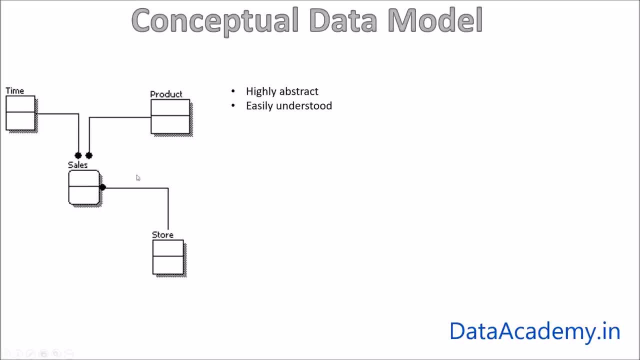 when we say abstract, we refer to the, to the fact that we do not have too much details right it. it is at a very high level, hence we call it highly abstract. it is easily understood. so whether the user is a technical or an untechnical person, it's anyone, for it's easy for anyone to understand what this model is. 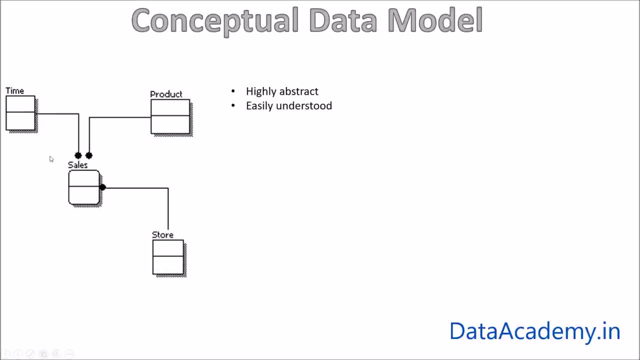 about. so, as you can look at this diagram, it's easy to say that there are four main entities: time product, sales and store. and all of the all of the three entities, which is time product and store, the information that is declared in theährt item, vaccines, which is Therapy. 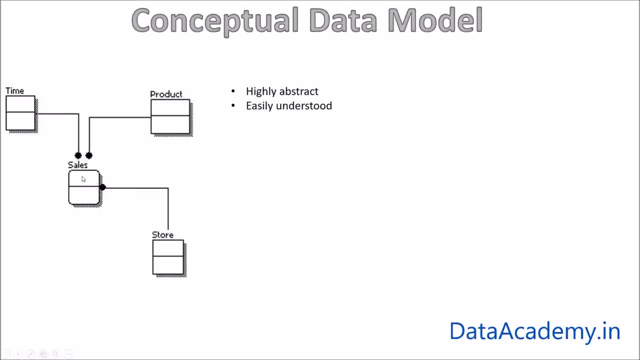 product and store have a direct relationship with the sales entity, right, so that way, there is a lot of information that can be easily obtained by looking at the conceptual data model, and since it is not a digital document, it can be easily enhanced. and the thing to notice here is: only the entities are. 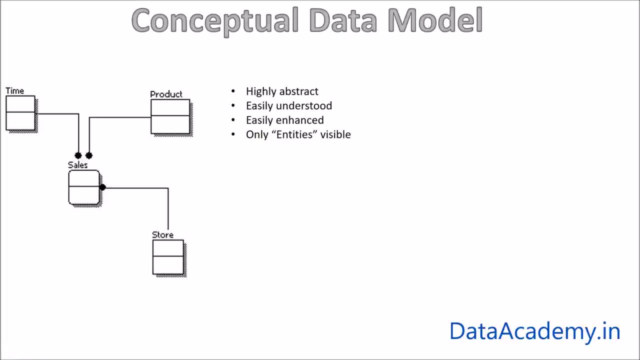 visible. there is something else called as attributes. those are not visible, but we'll be talking about it in just a bit. and even the relationships are quite abstract, meaning we just know that the product is connected to sales, but what is the column on which the relationship is established? that is not clear yet. so 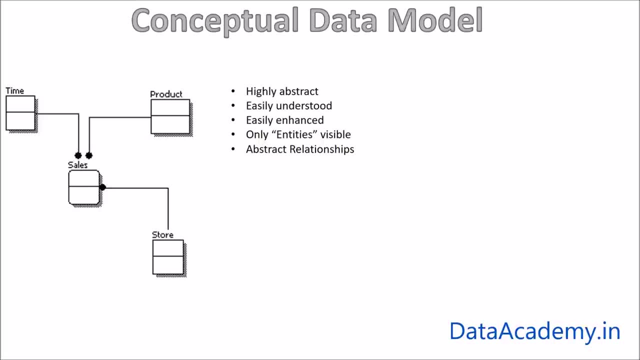 this is a way of hiding the complexity at at the very initial stages and since a conceptual model can be written on a piece of paper or a whiteboard, you really do not need, you really do not need a software tool to create a conceptual data model. that makes it a whole lot. 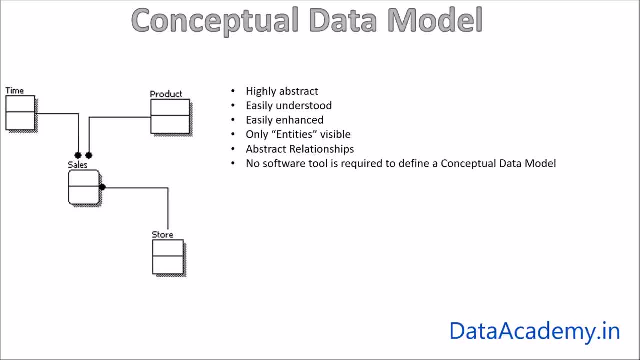 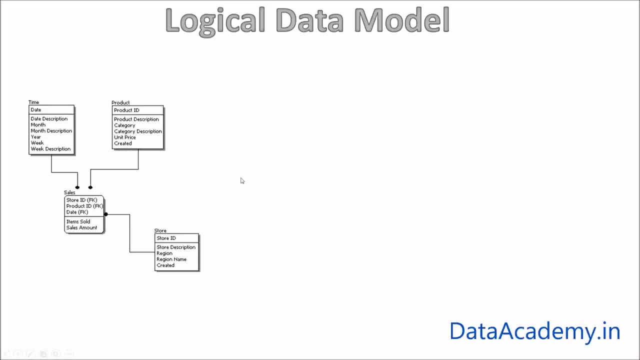 easier. once the conceptual data model is finalized, we can elaborate it into a logical data model. so let's look at a logical data model. so logical data model expands the conceptual data model by adding more detail to it. and what are those details? so first you'll notice, is the presence of attributes earlier. what 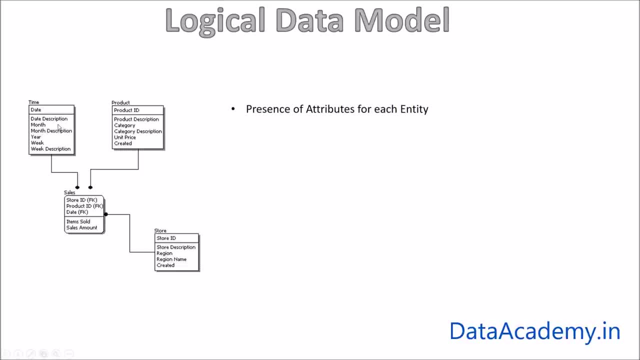 you used to be a simple square shape, now has a list of attributes. these attributes are further identified as key attributes and non key attributes. so key attributes, or attributes that define the uniqueness of that entity, such as in the time entity, it's the date that's a key attribute. similarly, we have 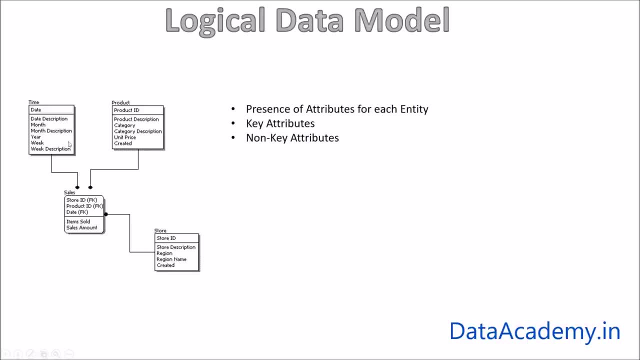 product ID for product and store ID for store right. so in the logical data model you draw a line within each entity. all the attributes mentioned or displayed above the line form the key attribute and all the other attributes below the line are called non key attributes, meaning they do not help in uniquely identifying a record. 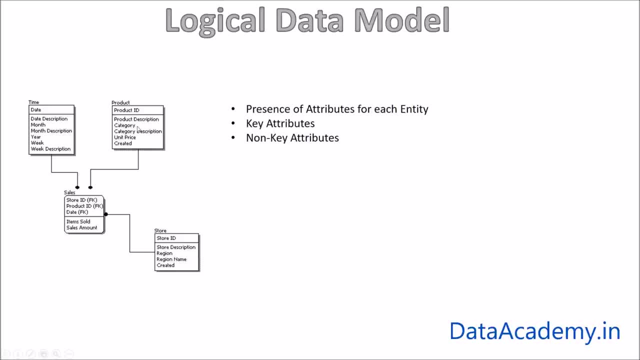 an example is the category in the product entity. so category is something that could repeat for a number of records. hence it's a non key attribute and that is why it is listed below the line in this entity. then we have the primary key- foreign key relationships- clearly defined, so the key attributes that are mentioned here for each entity. 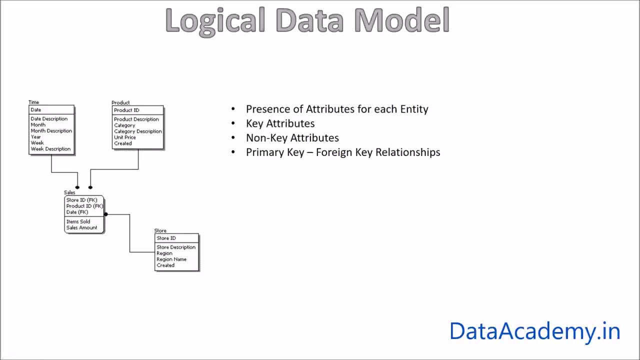 can also be used as a primary key and these primary keys are referred as foreign keys in the sales entity table, as it is apparent from the word FK enclosed within parenthesis right. so this is a detail that has been added and this was not available in in the conceptual data. 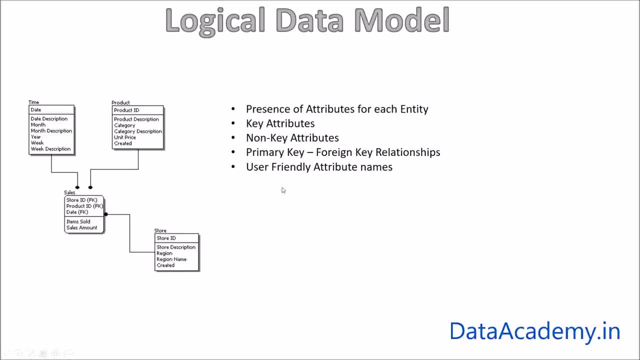 model. the other thing to notice is the user-friendly attribute names. right, so these are very easily readable. right again, any technical or non technical person can easily understand what each of those entities means. and to help to help in the readability, we have also given a single character space between: 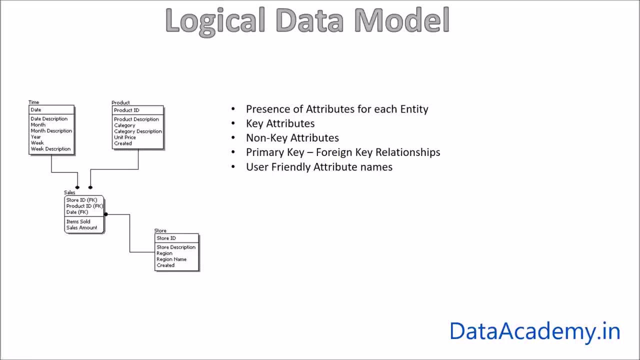 each word right and these words are by the dictionary, so it makes it very easy for anyone to read and understand and doesn't take too much time to to to understand what each column means, because they are self-explanatory and, given all these changes that we have done or or new things we have added to. 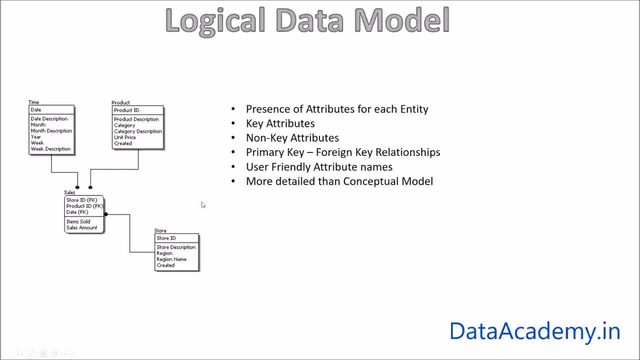 the logical model. it makes it more detailed than the conceptual model and, at this stage, this logical model is not dependent on any specific database, meaning you can take this logical model and you can implement it in any database. it may be Oracle, it may be SQL server, it could be even OLAP tools such as SQL server. 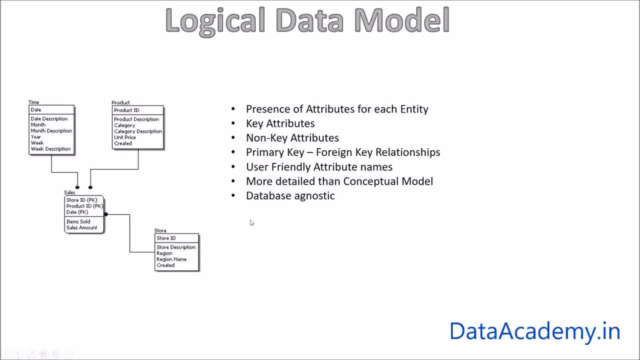 analysis services and so on. right, so at this stage it can be really converted to any database type. so that's the meaning of the word database agnostic, meaning it is not specific, rather it is generic. now that you have added all these details, starting from the key attributes, 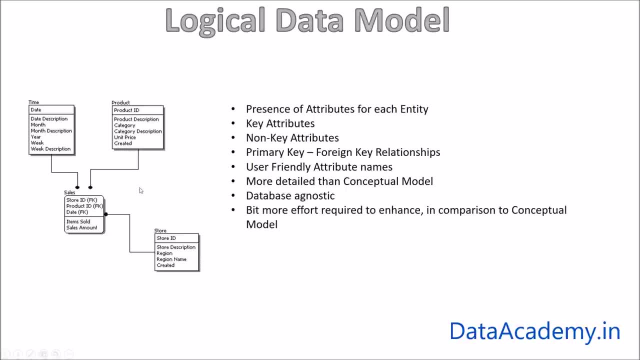 non key attributes, relationships, primary key, foreign key and so on. given all this, it makes it a little more difficult to enhance if there are any change in comparison to a conceptual model right, and this is usually implemented using a software tool such as Erwin or power designer. so these are tools that help. 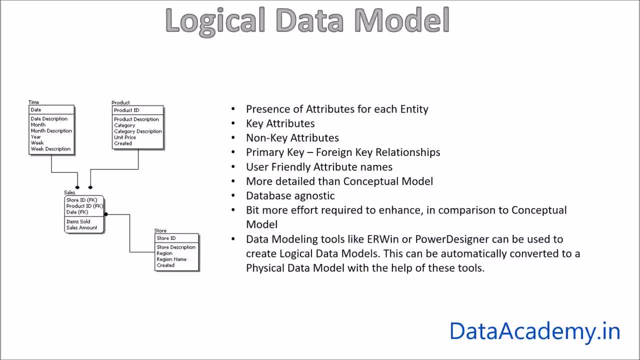 you define a logical data model which you can share, you can continuously update, and then you can- you can convert it into a physical model as well. so we will look at the physical data model in in just a minute. so, given all these additional properties of a logical data model, it makes it slightly more. 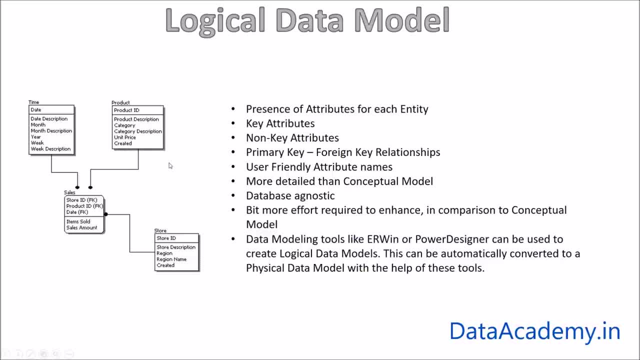 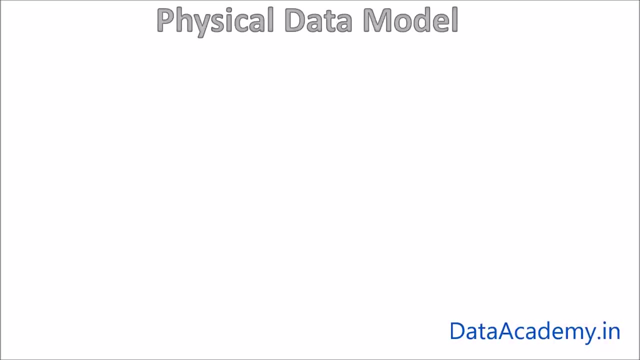 difficult than a conceptual model to update. once you have finalized the logical data model, we go to the last step of a data model design, which is a physical data model. so a physical data model looks little similar to a logical data model. however, there are some significant changes. okay, so to begin with here we don't refer to 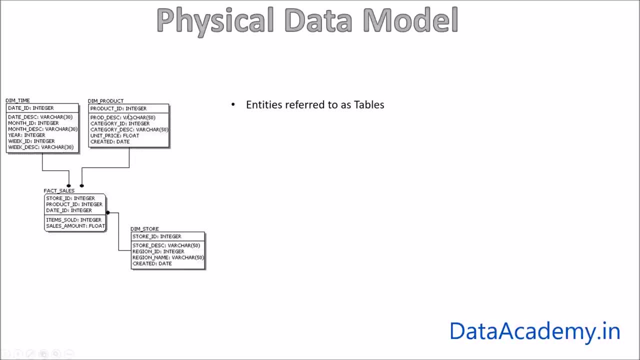 the entities as entities. instead we refer to them as tables, and what we used to call as attributes in the logical data model now we refer to as columns. So you see, tables and columns are words specific to a database, whereas entities and attributes are specific to a design, a logical data model design. 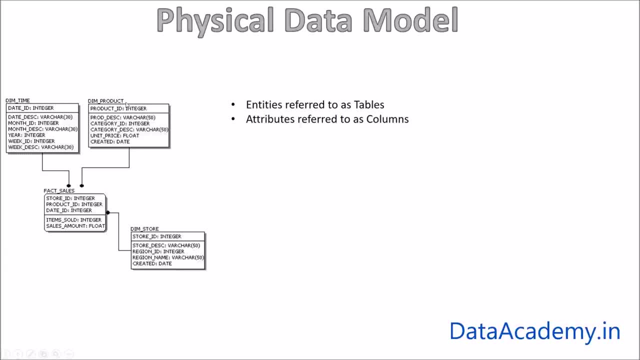 So when we create a physical data model, we should clearly be referring to these as tables and columns. The other thing that you notice is the column names. These column names are no longer user friendly. instead, they are database compatible names. so if you have worked on a database, you know. 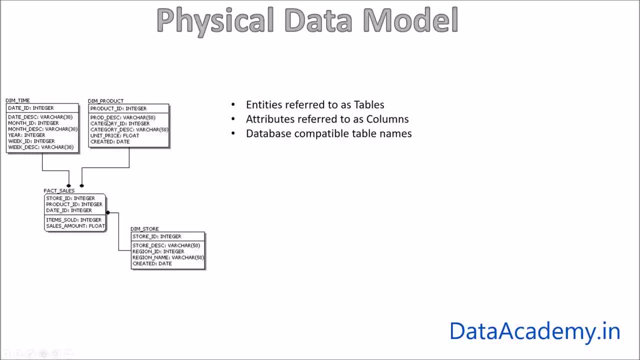 that, as a rule, you do not use a space when naming a table name or column name. although you can use a space, it becomes very, very difficult when you're writing queries using those list of tables and columns right, and hence you avoid using any special characters or any space between the words. 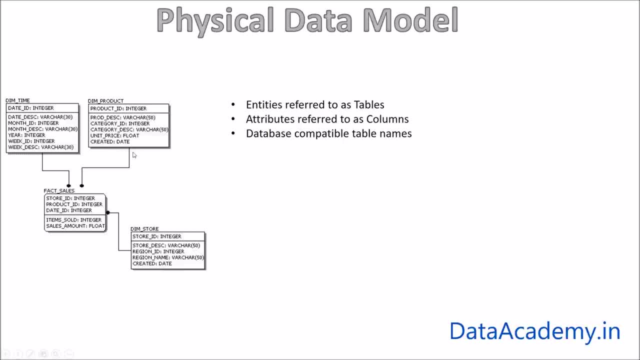 and one other thing that we do is we try to keep the column length as minimal as possible. so, as it's evident from here, for product the short form is prod. so product description has is now replaced here with prod, underscore de sc. right, so these are. these are database compatible. so this makes the life of a DBA. 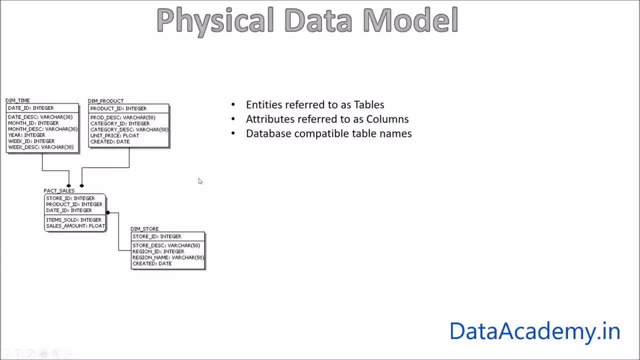 a lot easier by using names that are fully compatible with the database as well as any queries that we are going to write. so the same applies for the table name as well as the column name, and now we have introduced the concept of a data type right, so these data types. 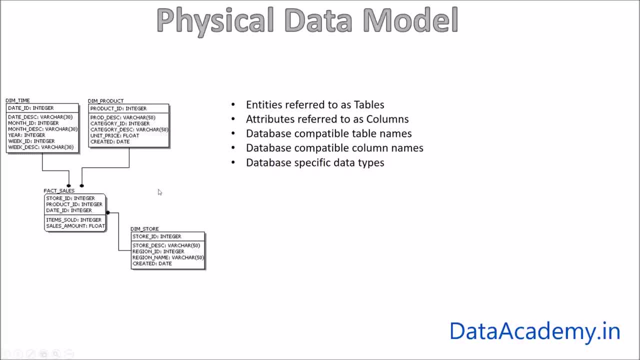 mention what is the type of data that's going to be used for the database. These data types are the types of data that are going to be used for the database be stored in every column. so, as you can see, here we have where care we have. 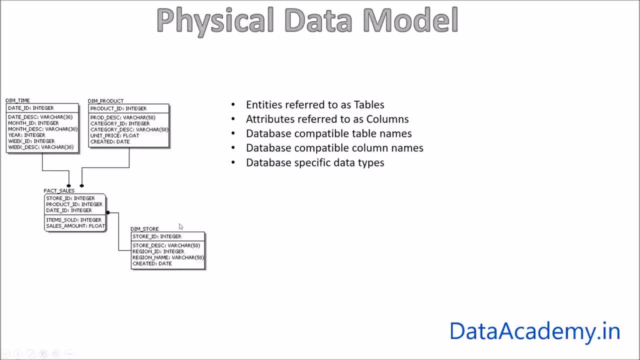 integer we have float, date and other other different other data types, so these data types are specific to a database. in this example, this physical data model is created for sequel server, which is the Microsoft sequel server database, so these data types are specific to sequel server. if you were creating a physical 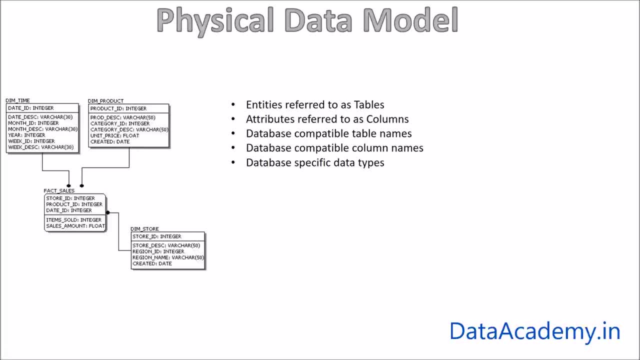 data model for a different database, such as Oracle or MySQL. these data types would be different, hence a physical data model is specific to a certain database. now, this makes it difficult for users to understand, so if you are talking about non-technical users, they will have a hard time understanding what each of 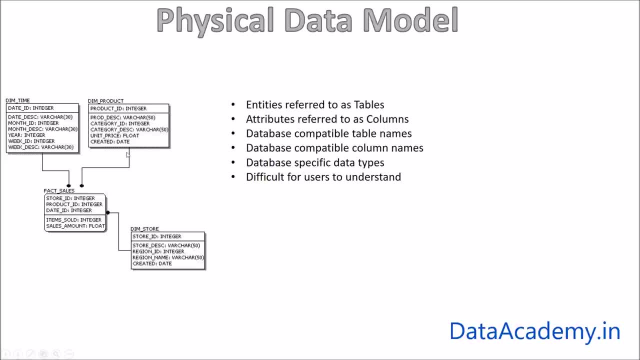 these tables mean, what of what these columns mean and what are these data types for? right? so it's a usually you. it's not recommended to share the physical data model with the users. you only share the logical data model. you, since this is this- has more details than a logical data model. it makes it even. 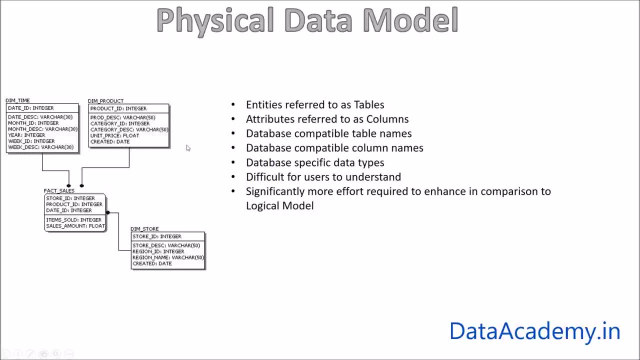 more difficult in order to enhance in comparison to a logical model. so let's assume that you a sign off on the logical data model and you go ahead and created a physical data model for a specific database. now, if there are any changes, you first need to apply those changes in the logical. 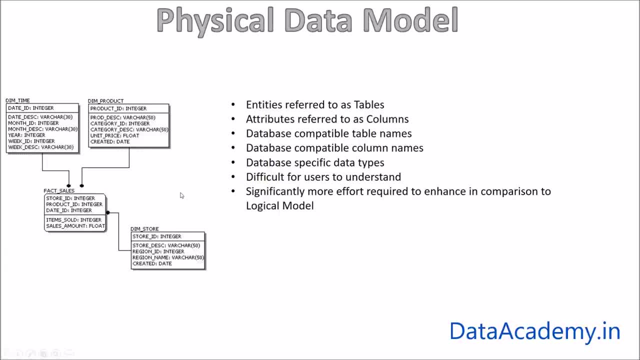 data model and then to the physical data model. so that's one kind of change which will take time. the other changes, let's suppose the database itself changed. now you're thinking of implementing this entire data instead of sql server, which means a lot of effort has to be involved in. 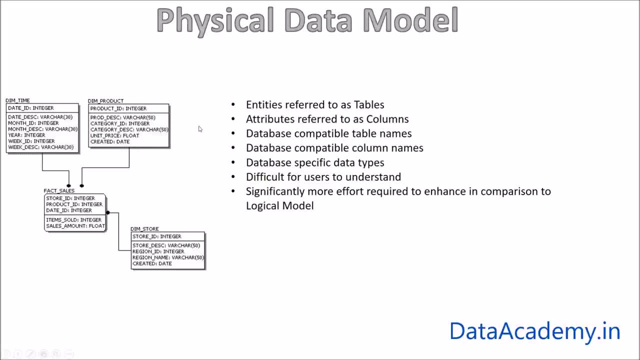 converting these data types to something specific to teradata, right. so that is where we have tools like erwin and power designer that will help you in automatically porting over the data, or porting over the logical data model to a physical data model of a certain type. and when it comes to